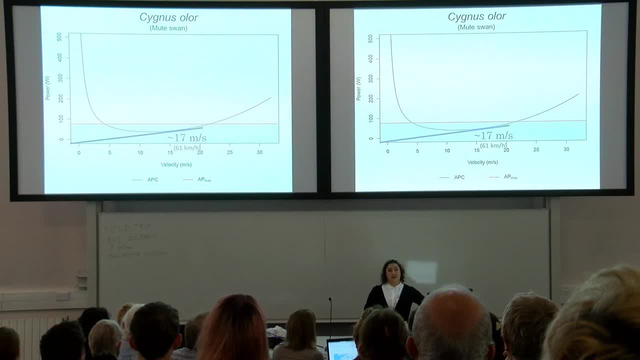 travel further, or its migration speed, And I can also tell you that a swan isn't very agile based on the relatively small power surplus that it has. Now, all of these stats that you've just seen are actually fairly spot on for a mute swan, So I'm sure you 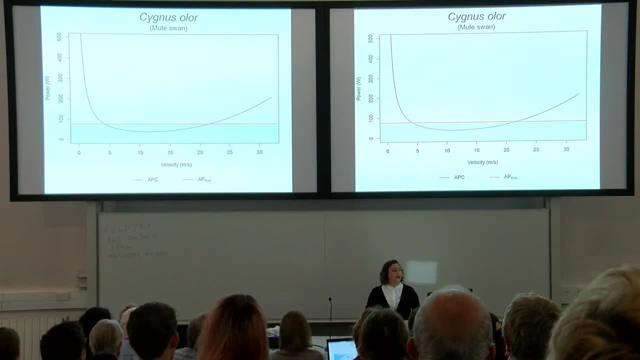 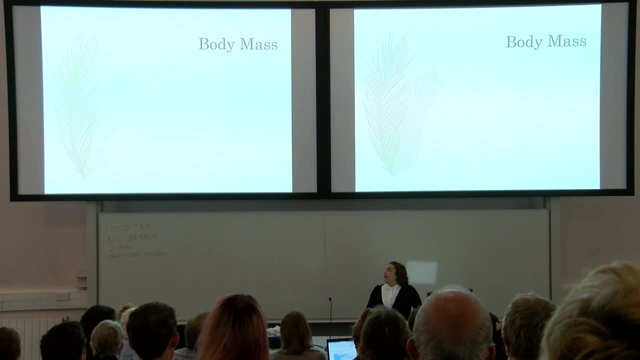 can see just how useful this could be if we could apply this back to the fossils. However, it's never really that simple in paleontology, now is it? So in order to find an APC, we need three measurements: Body mass, the surface area of the body or body frontal area, and 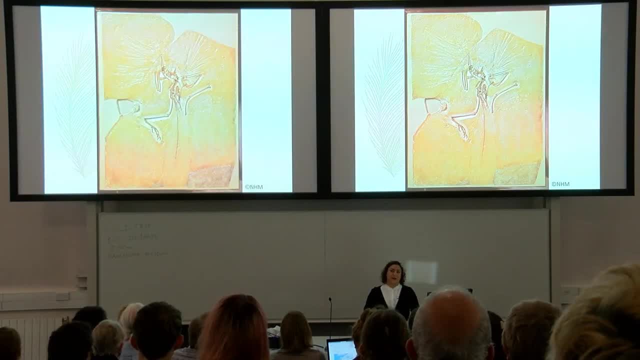 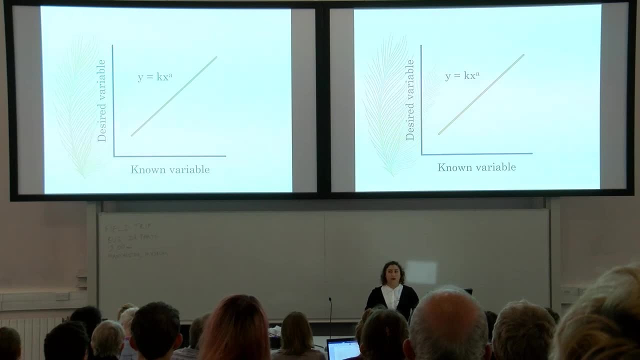 the area of the wings or wing area, And good luck getting those measurements from a fossil like this. Now you're going to tell me that the solution to my problem is using a regression equation to estimate the variable that I want, using a variable that I already have. Great, 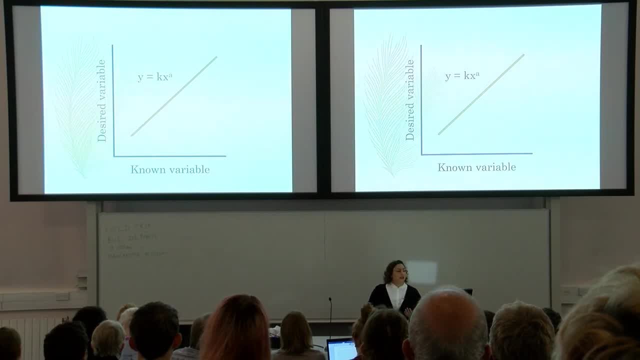 But there's one problem. See, there's an inherent amount of error associated with regression equations. that must always be taken into account, Whoops. And the way that we normally take this error into account is through confidence intervals. Now confidence intervals show. 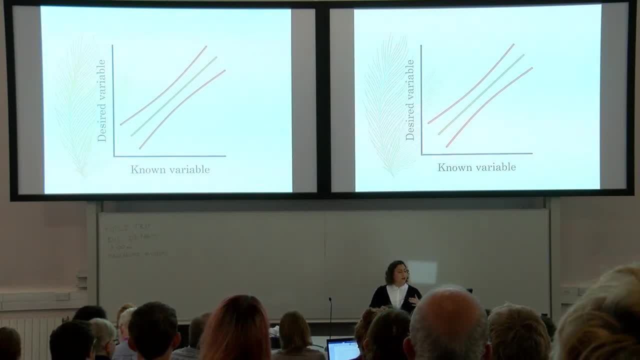 you how close your estimation will be to the sample, And the way that we normally take this error into account is through confidence intervals. Now, confidence intervals show you how close you are to the sample mean or the regression line, And this is a problem. 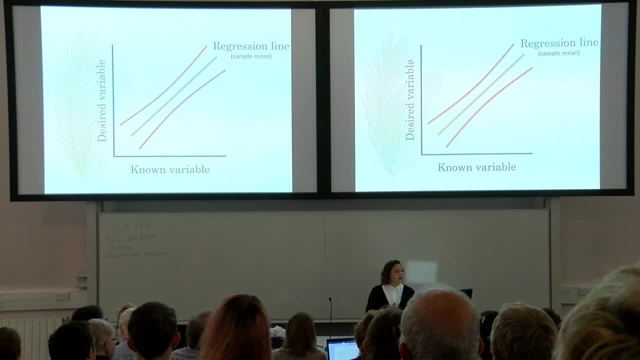 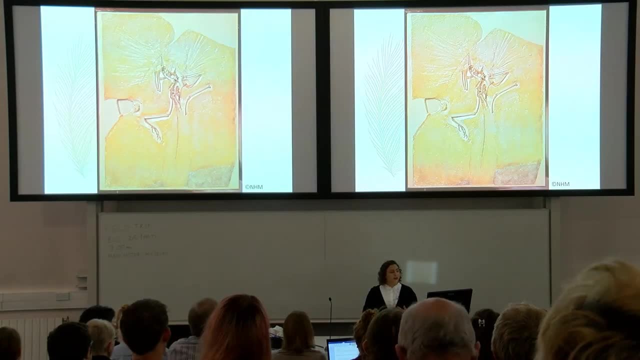 because our sample can only be made up of modern birds, so we can estimate the desired variable and the known variable in the first place and actually create our regression equation. However, as we all know, fossil birds do not necessarily have a modern analog, So that 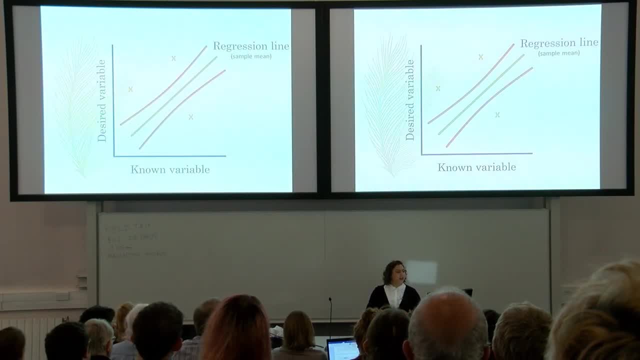 means that the true values of the fossil birds might not lie anywhere near this regression line showing you our sample mean. So that means our confidence intervals are out, because they might not actually cover where the true values of the fossils lie. So what we need instead are prediction intervals. 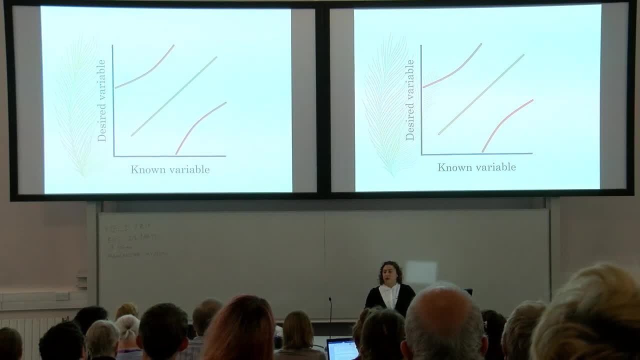 Now. prediction intervals are very similar to confidence intervals, but they're wider Now. they're wider just because they cover 95% of the data points within the sample and not just the sample mean. So that means that if you've constructed your data set well enough, then these should be representative of the entire population of birds. 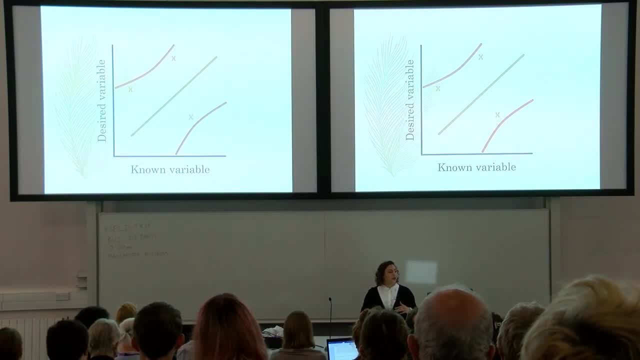 And then maybe, just maybe, it might also cover where the true values of the fossil birds lie. So we're already increasing the amount of error by having to use prediction intervals instead of confidence intervals. But that's not our only source of error, of course not. 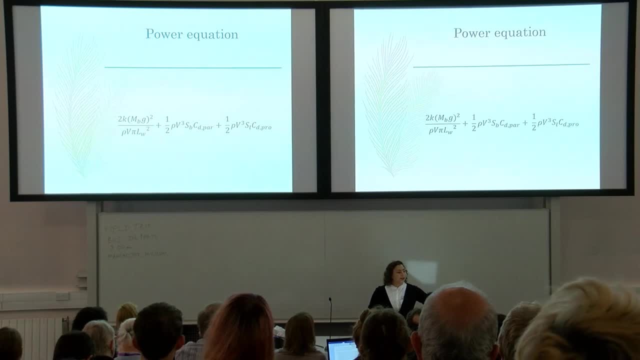 So the other source of error comes from the power equation that we have to use in order to calculate the APC in the first place. So the problem that we have here is that body mass is squared, and then both body frontal area and wing area are then added on top of this. 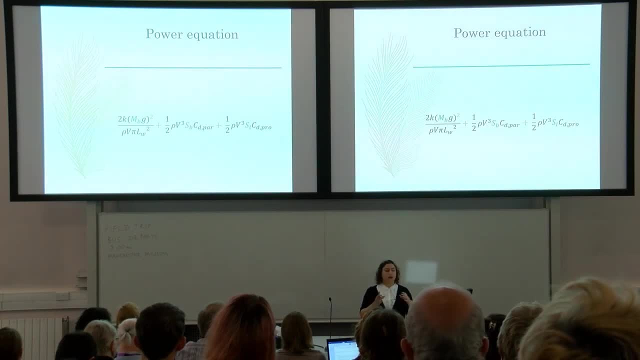 So what you have is the errors from multiple different estimations being combined all in one equation, And this is a phenomenon known as error propagation. Now, error propagation has its own specific set of rules that you have to follow, telling you how to do it. 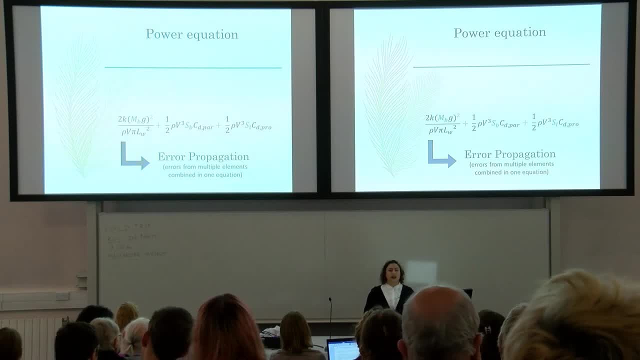 So you have to combine the errors from multiple different elements when they're all in one equation, And let me tell you, it's not as simple as just adding them all up. I really wish it were. Instead, there are specific set of formulae that you have to follow, telling you 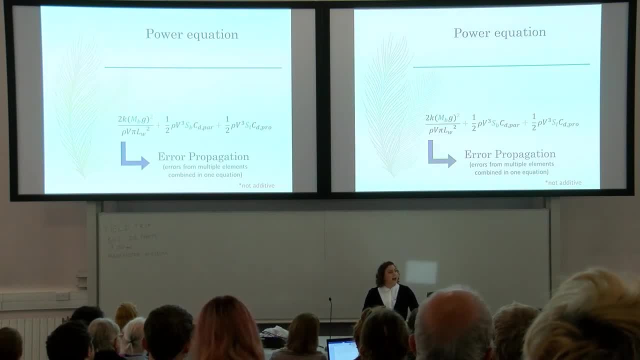 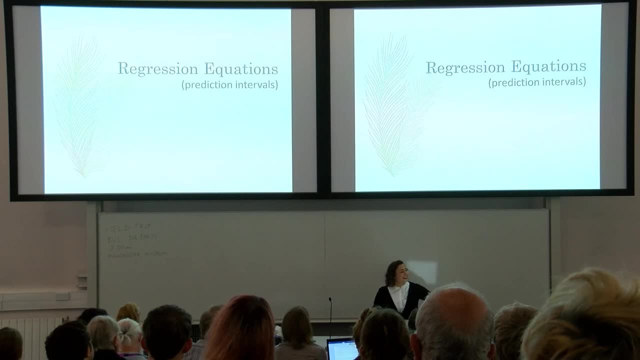 Sorry. there are specific set of formulae that you have to follow, depending on the mathematical signs and power levels within your equation, And overall this increases the amount of error present, because of course it does, So we have two sources of error. 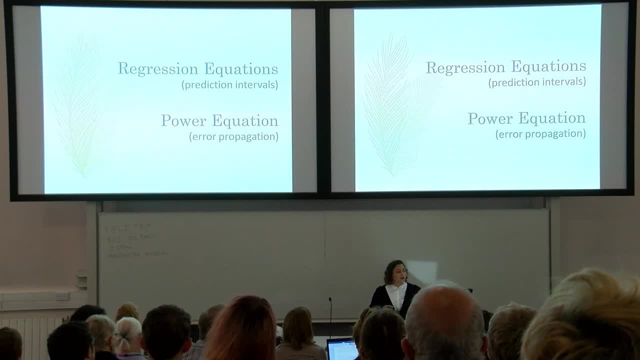 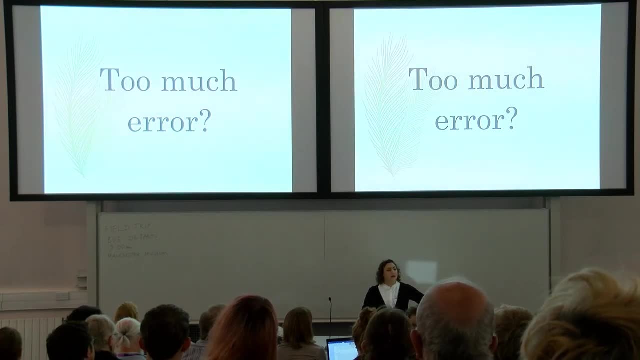 One from the regression equations and the other from the prediction intervals and error propagation. So the real question is here: is this actually too much error? Is there so much error associated with calculating an APC using regression equations created from modern birds that they've just become completely unreliable? 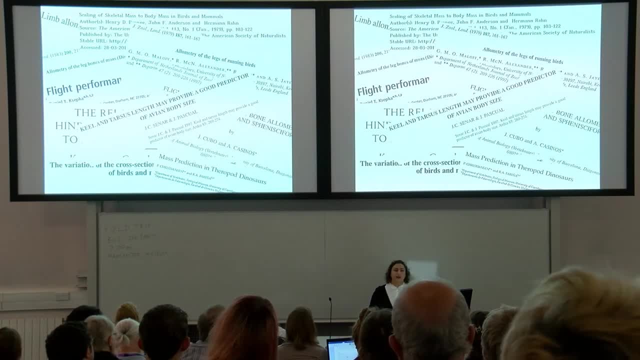 Well, in order to answer this question, I trawled through the internet trying to find as many regression equations as I could and data sets as I could for body mass, body frontal area and wing area, And then from there, I calculated their prediction intervals. 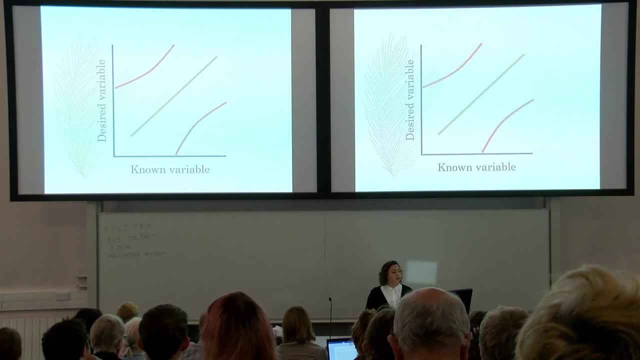 In order to compare all of these prediction intervals and see which one is the narrowest, I decided to find the relative width of them by calculating the percentage difference between the upper prediction interval and the regression line. I then used this value to find the narrowest prediction intervals. 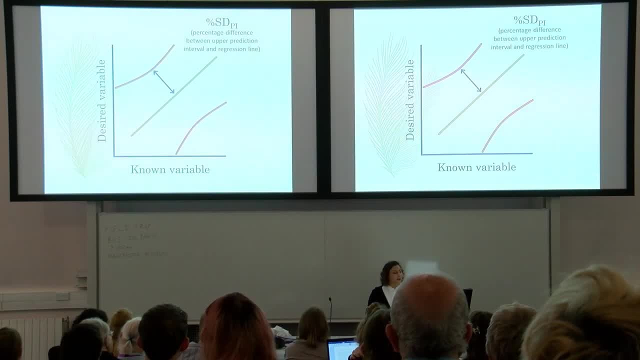 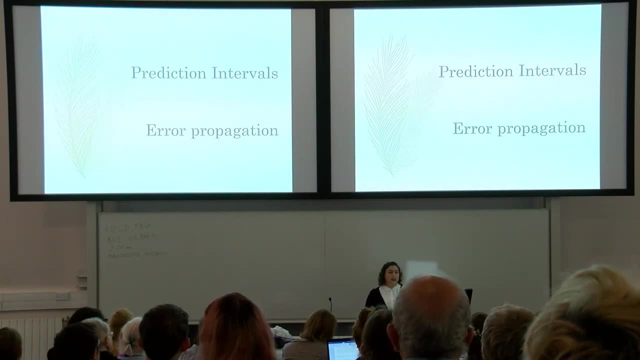 ie the regression equations, with the least amount of error, you know, to give this the best chance possible. And then, once I'd done this, I calculated some APCs and incorporated the error from the prediction intervals and the error propagation rules into them. 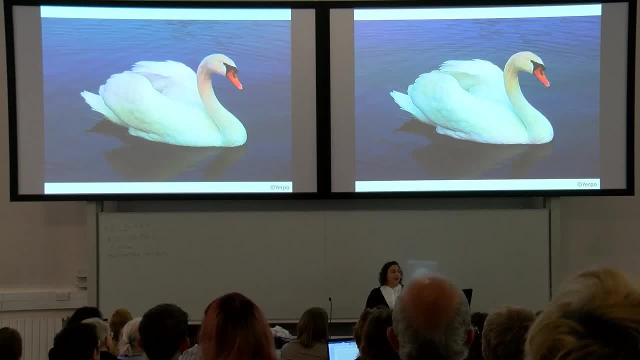 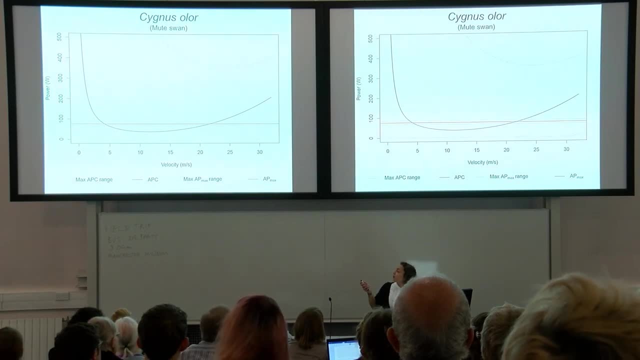 So, in order to see what the result was, let's go back to our mute swan. So this is the same chart that I showed you earlier, with the solid blue line showing you the, with the solid blue line being the APC that I calculated directly from the regression equations. 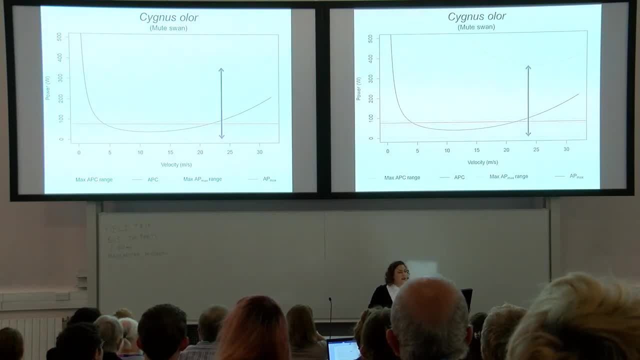 and this range representing the error margin. Now what I want to draw your attention to is just how big this error margin is. So, theoretically, I can have an APC like anywhere within this error margin and it would still be a valid result. 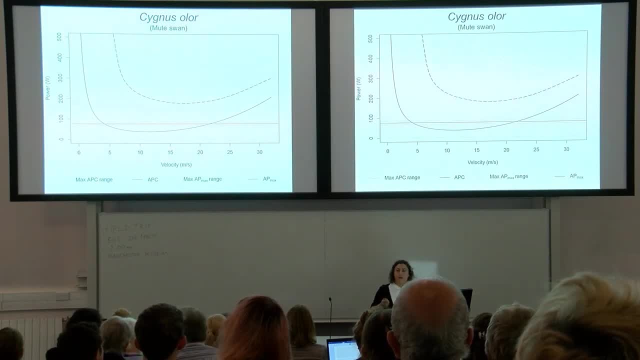 I mean, I could even have an APC, like all the way up here, you know, above my red maximum producible power line, which would mean that my swan couldn't fly at all, which is obviously a bit ridiculous. I mean, obviously swans can fly right. 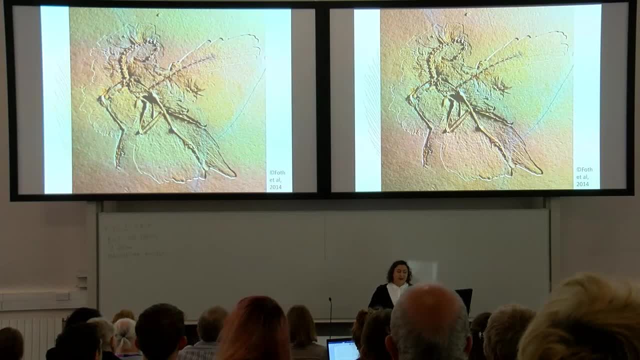 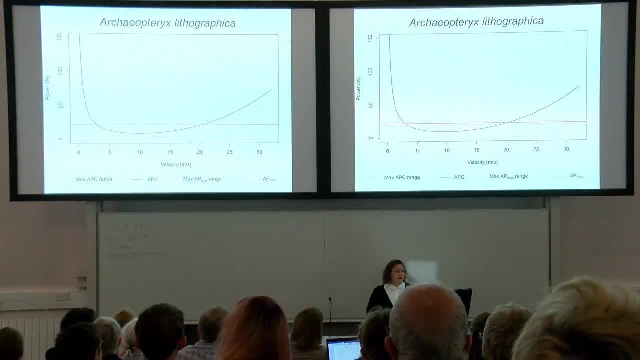 Well, yes, but can you really say that for something like Archaeopteryx? Not with any certainty. And lo and behold, if we look at the APC for Archaeopteryx, we have a very, very similar problem, whereby the upper limit of the range within which an APC can lie. 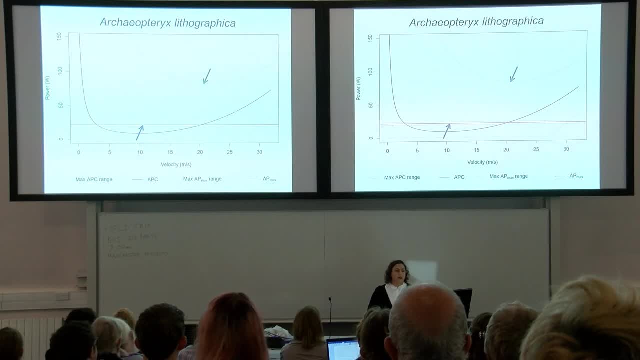 is way above my red maximum producible power line. So basically this means I can't tell you anything about the flight capabilities of Archaeopteryx based on this graph. I got nothing, So at this point I was almost ready to throw in the towel. 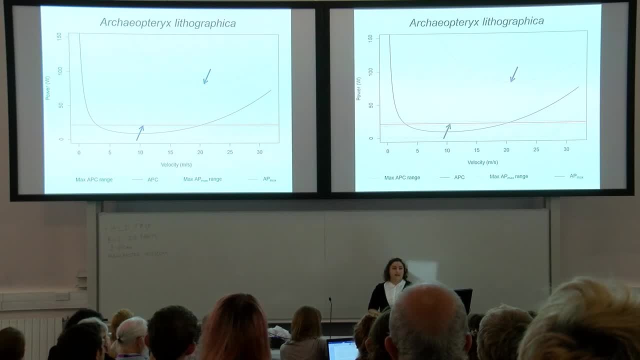 and just storm off in a rage, but then I calculated the APC for this specimen. So this is Salmila robusta, which is a Middle Eocene crane-like bird, and this is its APC. Now, what's interesting here is that our upper limit. 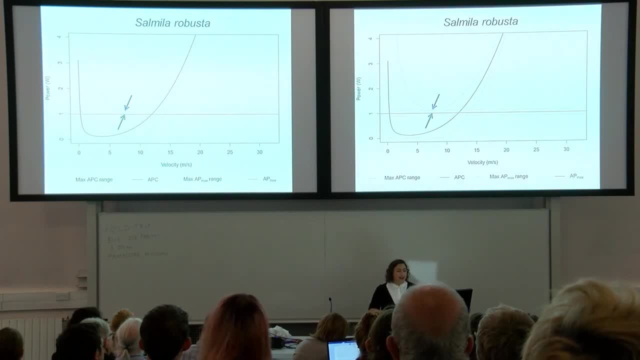 is really, really close to our maximum producible power line. I mean, it's not below the line, but you know it's getting there, which made me think: why is the error margin so different in this sample compared to the other samples? 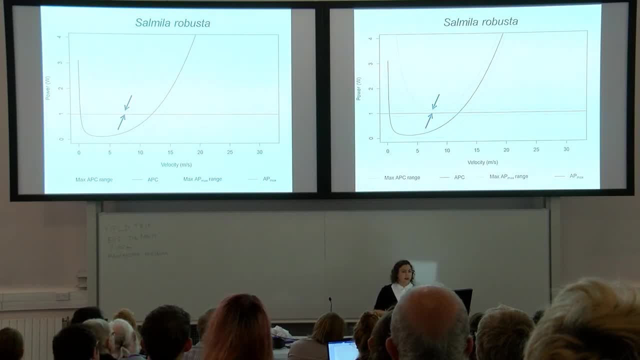 Well, in order to answer that question, I decided to find the relative width of the error margins as the percentage difference between the upper limit of the range within which an APC can lie and the APC itself, And then I correlated that value against my morphological variables. 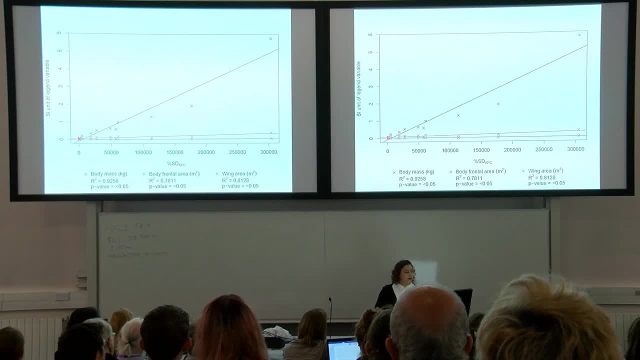 as in body mass, body frontal area and wing area, And this is the result. Now, what's interesting is that every single one of the morphological variables is strongly and significantly correlated to my range: width In particular, though, body mass has a particular 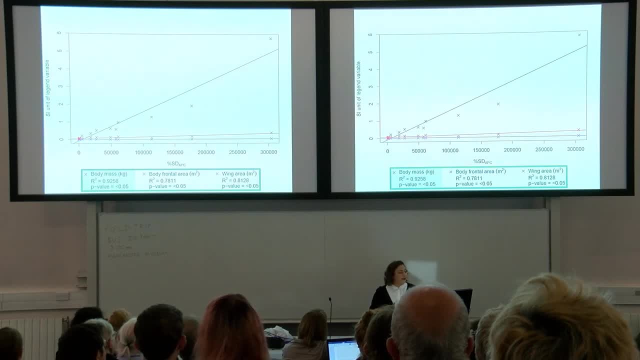 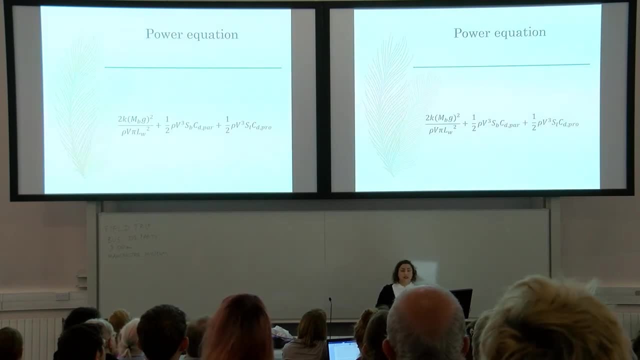 Hello. OK, In particular, though, body mass has a particularly strong correlation. So why would that be? Well, if we go back to our power equation, we can see why. So, as I said before, body mass is squared. 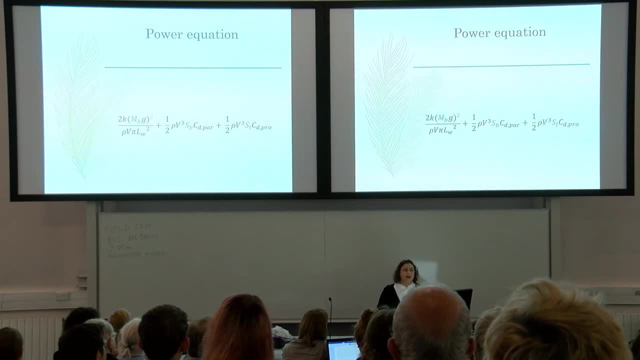 On the other hand, neither body frontal area nor wing area are raised to any power. So that means that any error associated with estimating body mass is going to be translated much more strongly into our APCs and is essentially the main reason for this massive error that's happening.